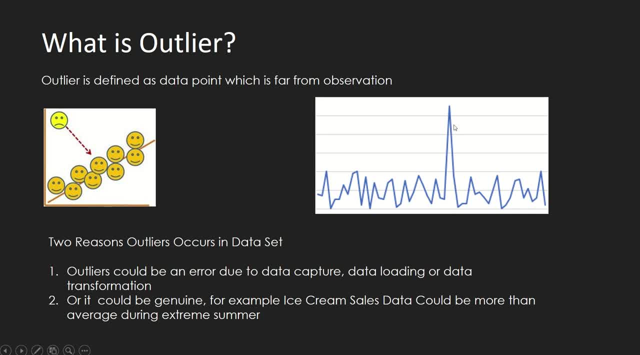 you have a 50% discount and because of that, the orders were too high on that day. Okay, So you can see on this day the orders gone too high and if you see, normally you will say that this is an outlier. But this is obviously it's an outlier, but that's a genuine outlier because of some business reason. 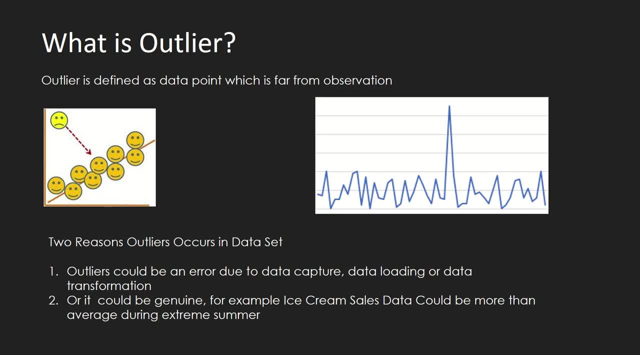 Okay, Business justification. So there could be two reasons for having an outlier in your data set. Okay, And based on the reason why outlier is there in your data set, you will have to deal according to that. okay, if the outlier is because due to some error, okay, then you will have to remove the. 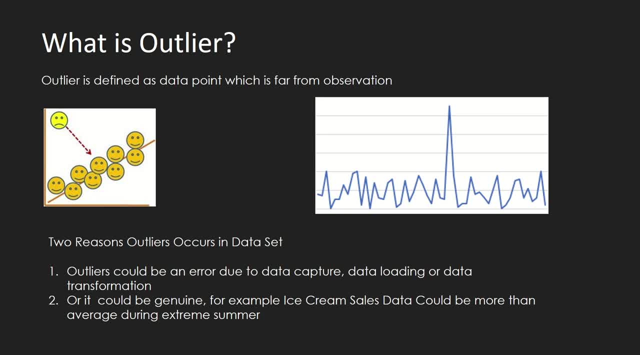 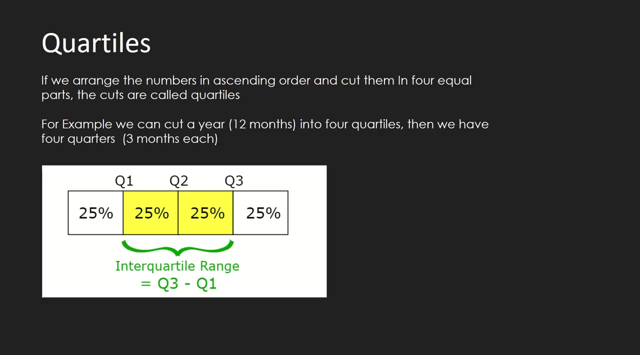 outlier and if it is because of some business region, okay, you might want to include that outlier in your analysis. but this tutorial is limited to understand how to detect an outlier, so let's go ahead and see. okay, first of all, we'll talk about quartiles. even before understanding box plug, it is important. 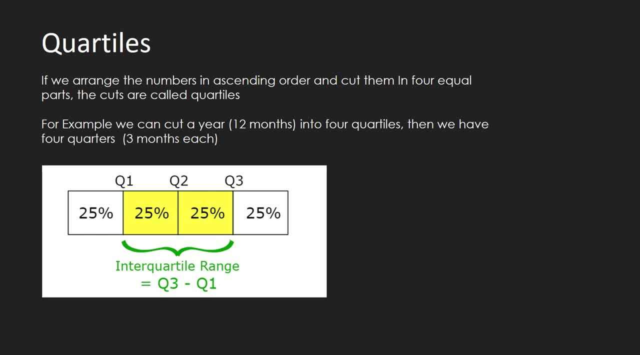 to require to understand quartiles. what is quartile? so let's say you are having a data set- okay, this is a data set- and I am telling you to divided that data set into four equal parts. now, in order to divide that data set into four equal parts, you will mark three lines there. 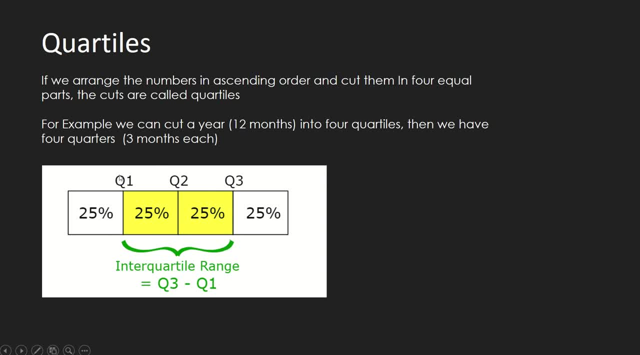 okay, Q1, Q2 and Q3. so if I draw three lines, my data set would be divided into four equal parts, parts 25 percent, 25 percent, 25 percent and 25 percent. now, each of these equal distribution is called quart quarters. okay, so this is a quarter, this is a quarter, this is a quarter and this is a 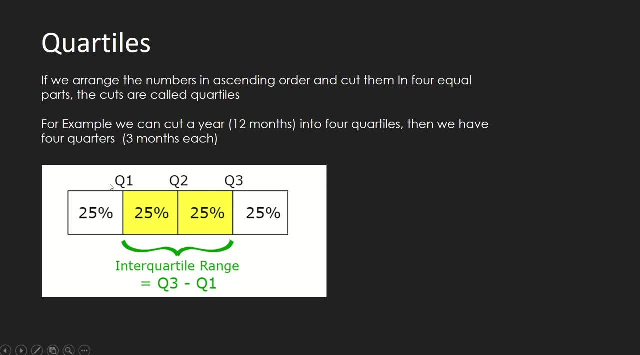 quarter. now the lines by which i am dividing the data is called quartiles. okay, so q1 is quartile, q2 is quartile and q3 is quartile. okay, and the middle one, middle quartiles. okay, like 25 percent. and this 25 percent which is highlighted into yellow, okay, that is called interquartile range. 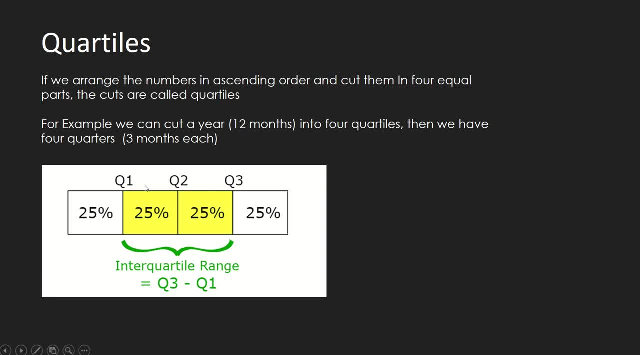 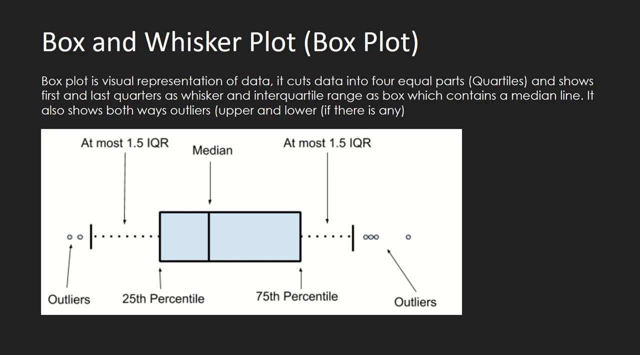 so q1 to q3 is interquartile range, because this is inside these boxes, this box and this box. so quartile and quarters are really important concept. before drawing a box plot now let's go and see what is a box plot. if you see block box plot here, it's not just a box plot, it's a box. 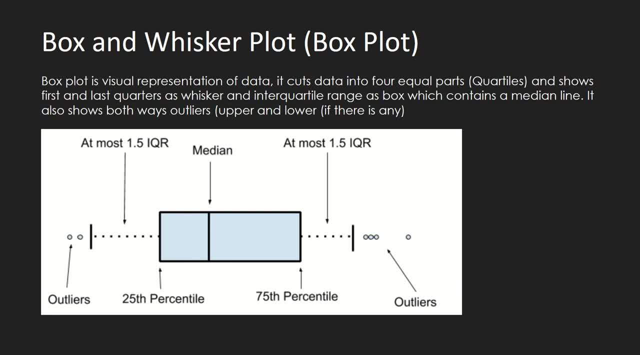 and whisker plot, but it is popularly called as box plot. now, what does it contain you? it contain a box. this is a box and two whiskers: the upper whisker and lower whisker. okay, if you see carefully, even this data set is divided into four equal parts. this is one, this is two, this: 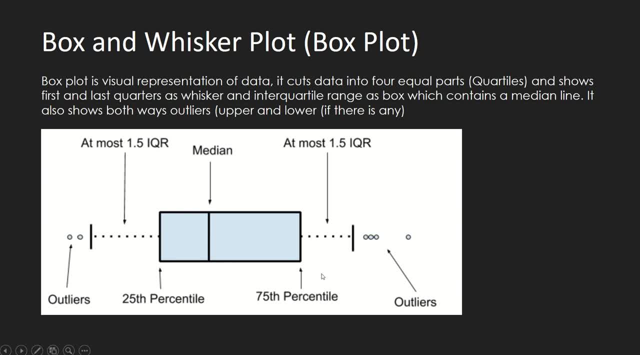 is three and this is four. okay, it even contains some outlier in your data set, okay. so if you see this point, okay, this is an outlier and this is an outlier. so box plot is visual representation of data. it cuts data into four equal parts, which is all based on the find into the eğa, so this square now together. it's shown in vídeos. 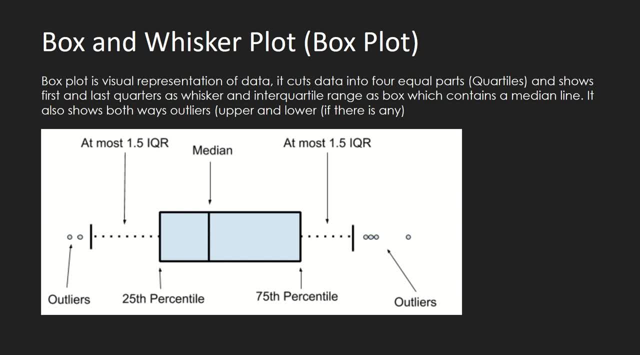 to chaos. captain level. i want you to see how design all this here. okay, so this is all- uh, as i said, it actually contains some idea as well- to everything. okay, so this one here is between h2 and h3. okay, so the first & the quarter is whiskers as well, and interquartile range as a box which contains a median line. okay, so, if you see, this isエqnQ1 mouse Location. after a box of those image dot will have the crocodiles symbol. 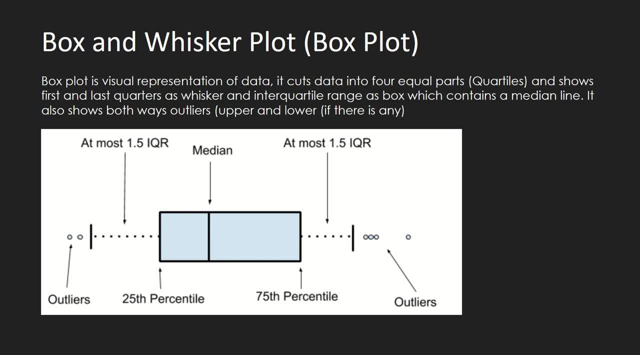 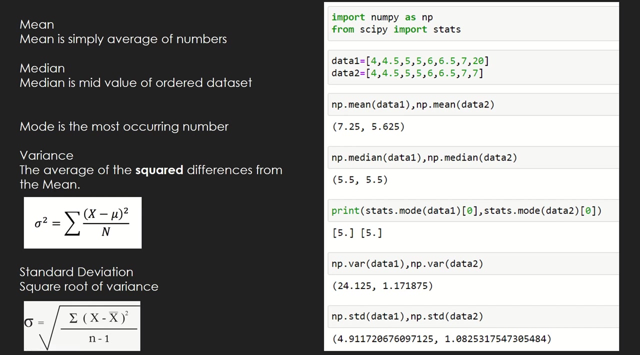 range q1 and q3 and this range contains a median line here, okay, or it also has the second ward and there are also. So this is all about box plot and whisker plot. We'll go ahead and see how to draw this box and whisker plot actually, But let's talk a little bit about ZS score. So we spoke about mean and median here. in box plot You can see median, But what is median? We'll talk a bit about that. Okay, So mean and median are basically same thing. It's kind of average, and even more is there. Okay, So mean is simple average of numbers which you are. 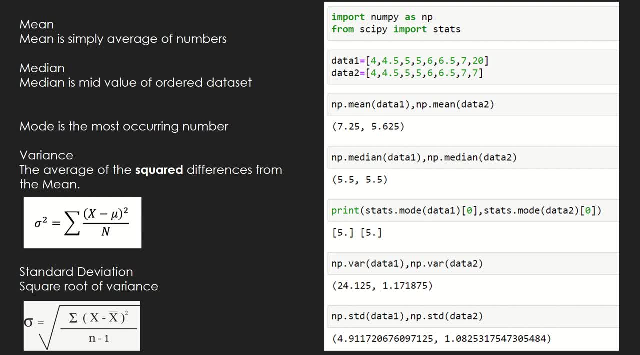 studying from your high school And median is the mean value when data set is ordered, Okay, And more is the most occurring number in your data set, Okay. So if you can see the data set here, I have took two data here, data one and data two, And this data is already sorted, Okay, And the mean of data one: data one contains a outlier, Okay, 20.. And data two doesn't contain any outlier, Okay, So the mean is 7.54. data one: 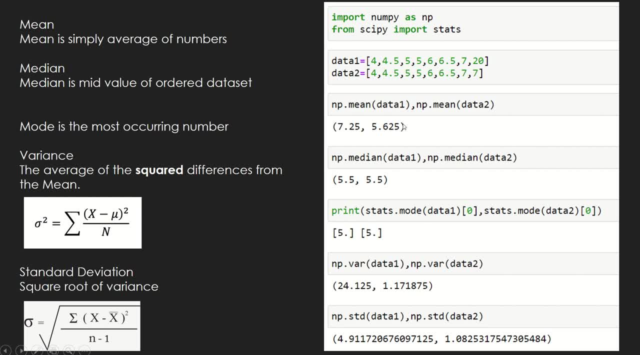 Because it has outlier and the mean for data two is 5.6.. Okay, So it means the mean is affected by having an outlier in your data set, Whereas the median because it is the mid value when data is arranged in some order- Okay, ascending or descending- So median remains same for both the data. So it says that, in case we think that there could be some outlier in data, talking about average would be good for median. 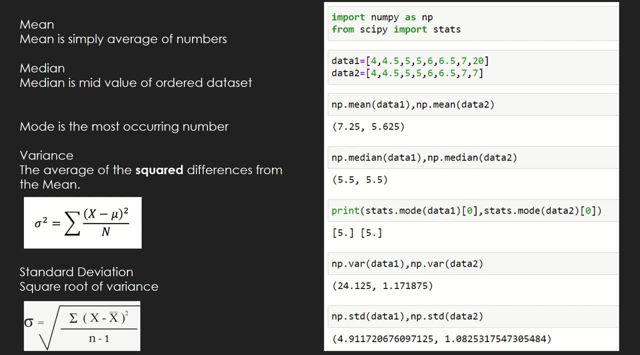 Okay. So rather than taking mean, we will take median in that case. Okay, Now mode is same thing: most occurring number. So in this data set, if you see what is the most occurring number: five, five. so five is occurring two times. So five is the mode for both data set. So whenever there is some outlier in data set, rather than taking mean, you should took, you should take mode. Okay, Now go ahead and talk about variance. So variance is everything. 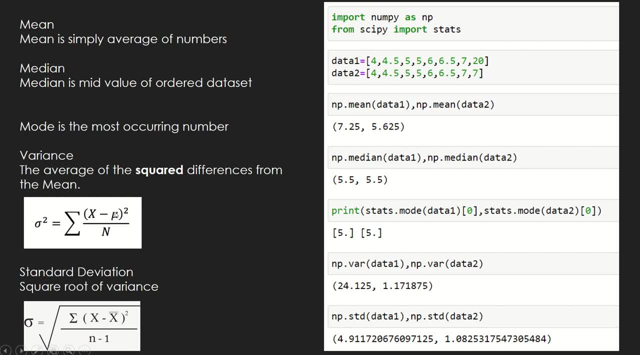 So the average of the square differences of the mean. So if you say this is the mean of the data, Okay, And this is my data point. So if I subtract my data point from all the data points, from the mean, and take a square of that- okay, and take the average for that- okay, some of the average, then that is called variance, Okay, And that indicates that how much variability is there in my data set. So that is important to understand using variance Okay. 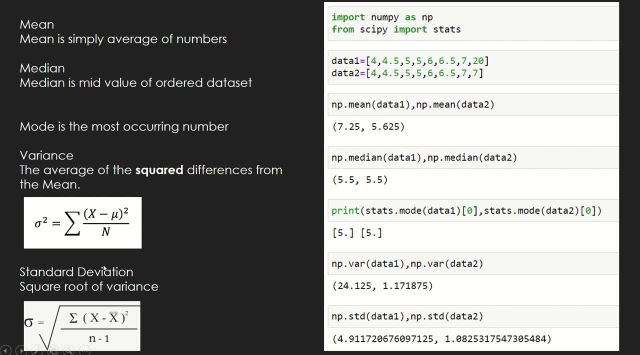 Now, since variance is a square of the distances, we can take a square root and that value is called a standard deviation. So a standard deviation is nothing but a square root of variance. Okay, We can find variance and standard deviation by using numpy, And we'll talk about pandas, data frame as well, in in five minutes or so. Okay, So see how we take variance- np dot var. Okay, And we take a standard deviation using np- dot standard. 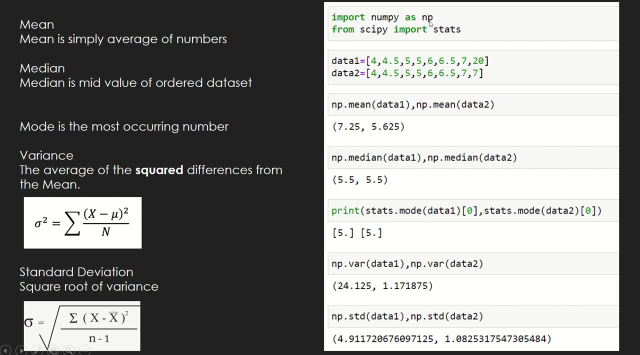 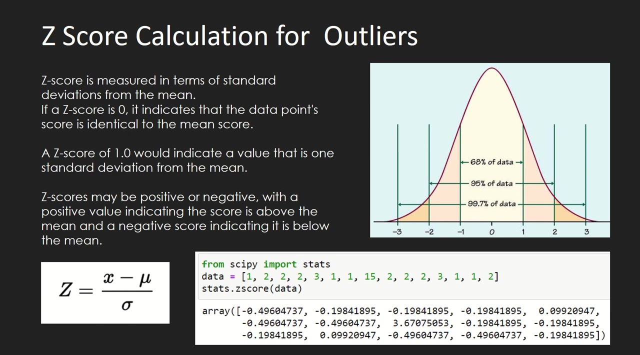 deviation, std. So that is from numpy package. Using numpy package you can take mean, you can take median and you can take variance. you can take a standard deviation, but there is no method for mode, I don't know why. Okay, So for that you'll have to import other package called scipy. Okay, Now let's proceed and talk about z score. So what is z score? z score is measured in terms of a standard deviation. Okay, So it is kind of a standard deviation only, But the value of z score would be. 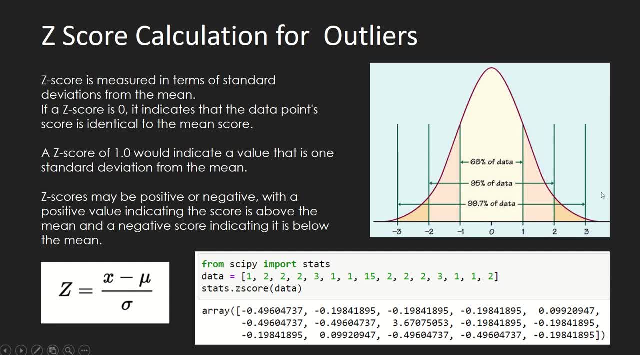 either minus one minus two, minus three, or one, two and three, So it could be positive 123 or negative 123. Now z score one: indicate that a value is one standard deviation from the mean. z score to indicate that value is to a standard deviation away from the mean. Now this is the mean line. right? This is a normal distributed data. Okay, Normal, because if you see, this is the mean line and the 50% of data is here And 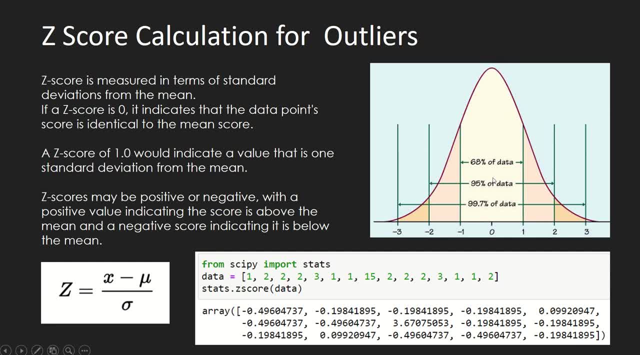 and 50% is here. okay, so this data is normally distributed, or we call this as bell curve. now, if you see z square 1, if you see this is 50%, sorry, 1 standard deviation away from the mean line. z square 2 is 2 standard deviation away from the mean line and 3 is 3 standard 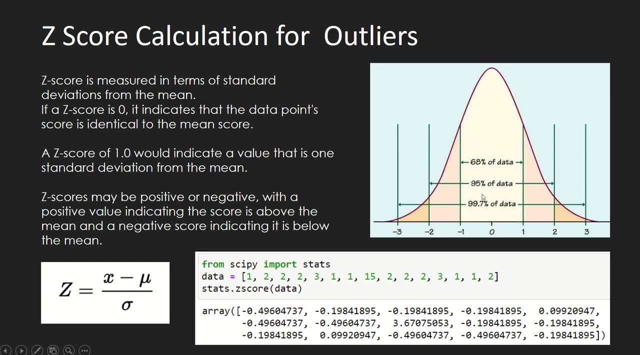 deviation away from the mean line. so that is about z square. okay, and z square essentially represents that: how much away is your data point from the mean value? this is calculated as the data point itself when subtracted from the mean value and divided by z square. okay, so that gives me the 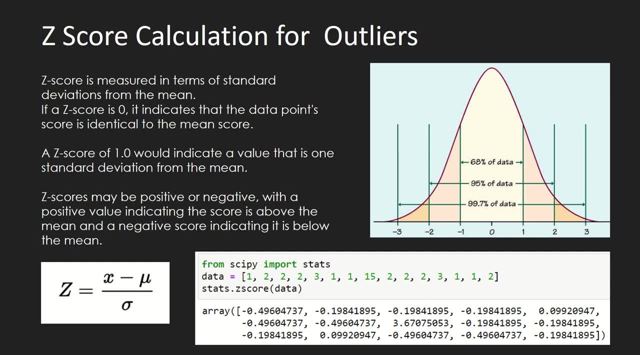 times number of times it is away from the mean value. great, now we can calculate z square by a stats package of psi, pi. okay, and you can see i have calculated a z square. it is said that if the z square of a data point is less than or equal to z square, then it is less than or equal to. 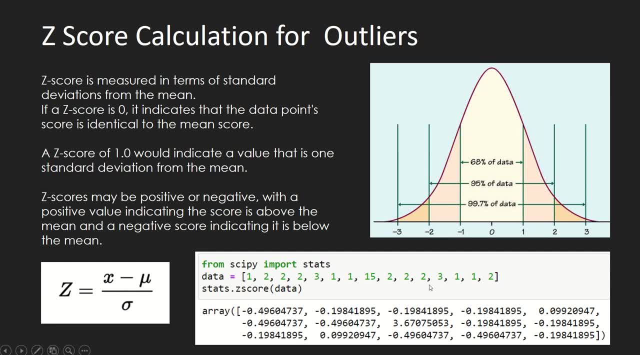 3. that point could be treated as an outlier, okay, so here in this data set you can see the z square for this number: 15 is 3, but rest numbers are 1, 2 and you can see 15 is far away from 1, 2 and 3, right, so this is an outlier, okay, and the z square value for this data point is: 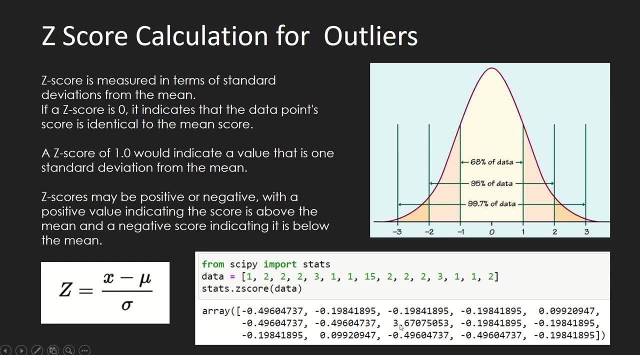 3.67, so i can treat this number as z square. okay, but there is no such hard and fast rule that, in order to be an outlier, the z square for your data points should be three or more than three. okay, based on your business requirement or threshold, you can decide the score too. 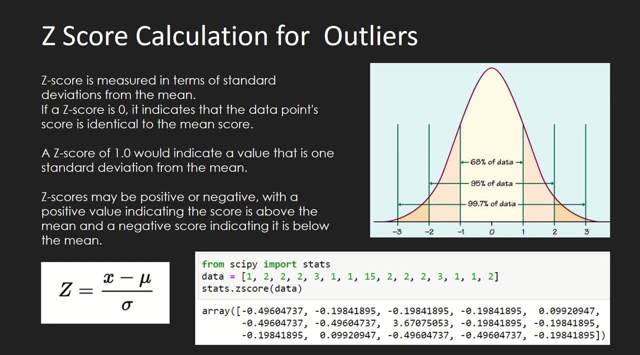 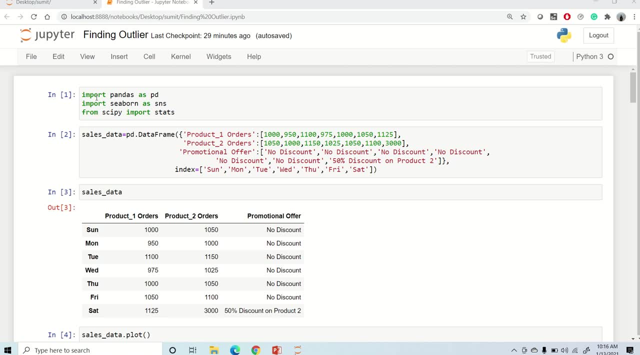 okay, or one point, five, five as well, okay, or even three. so that is dependent, uh, depending, on your business requirement. now let's go ahead and see implementation of all these things using python. so here i have jupiter notebook and we are going to implement z score and box plot using 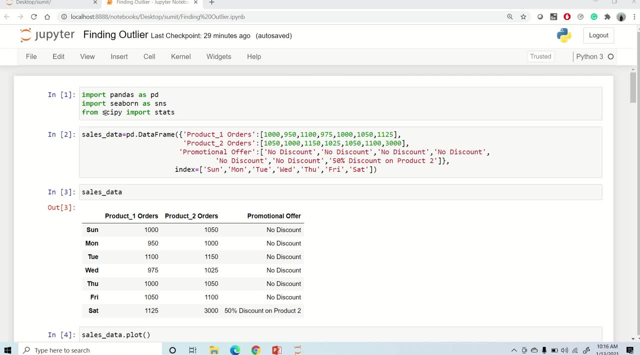 using python. we need pandas library, seaborn library and scipy library. now, just, uh, to tell you that you can download this jupiter notebook from the link which i have given in description box for your hands-on or practice. okay, so what i have done actually, here is created a data frame. 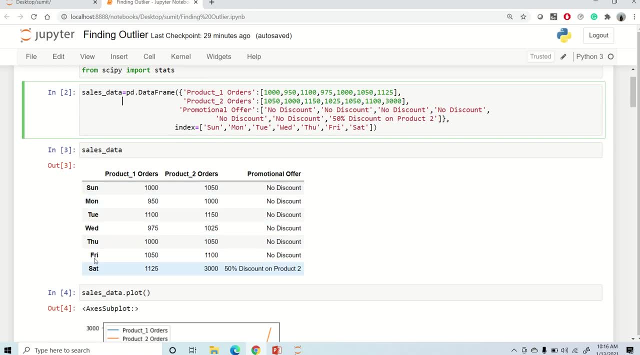 and this is, uh, some online sales data. okay, let's say online sales data for a week, sunday to saturday, and there are two products, product one orders and product two orders. so these are the orders for some products and, if you see, data are same for both the products. uh, just 50 difference in both. 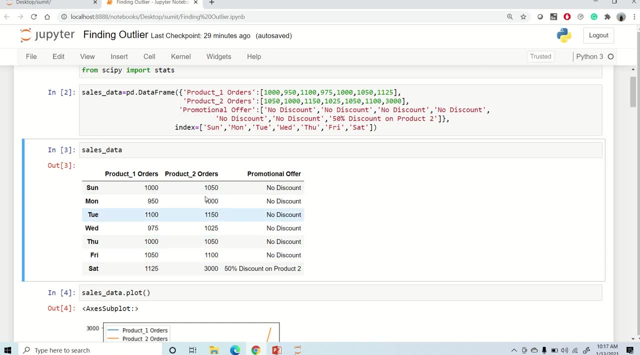 of these, okay, only product two is having some offer at the end of the uh week. okay, weekend offers, let's say, 50 discount on product two, and for that reason, the product two orders became thrice as normal, okay, on saturday. so this is our data set and i have created this data set. 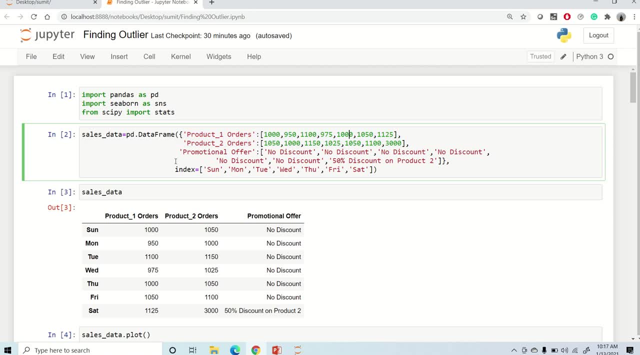 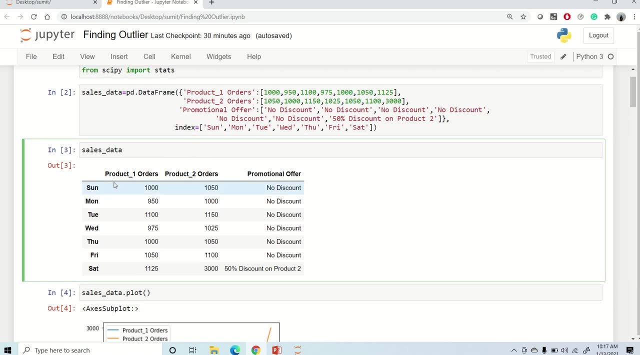 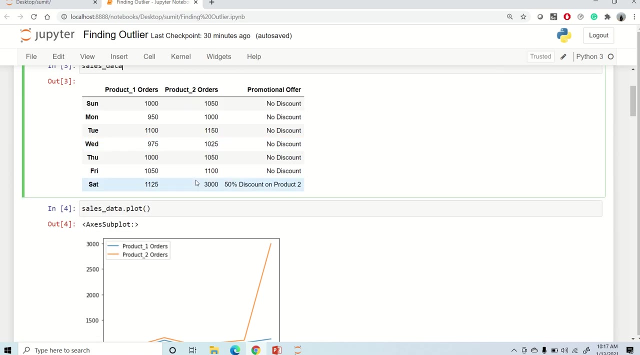 by you dictionary here, so you can manipulate this from the this code here. okay, and you can do some changes if you want. so this is how our sales data look like. and in order to identify the outlier, okay, first thing you can do is plotting a line plot. okay, so if you say data frame, dot plot. 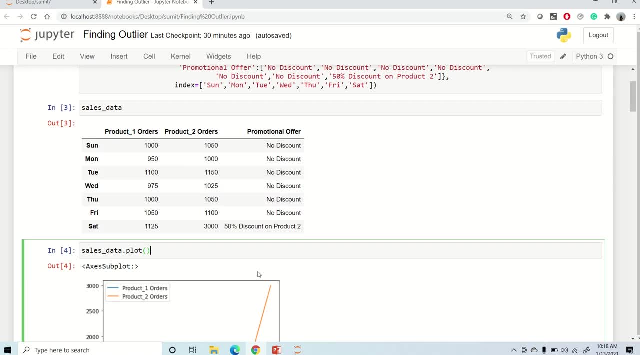 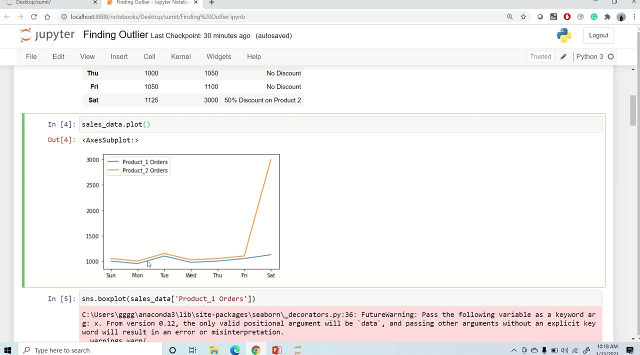 it will ignore all the string columns and will plot a graph for you for numerical columns so you can see product one and product two. sales look similar. okay, orders look similar, but only for product two. it went too high on saturday. okay, this point here, saturday, and it seems that this is. 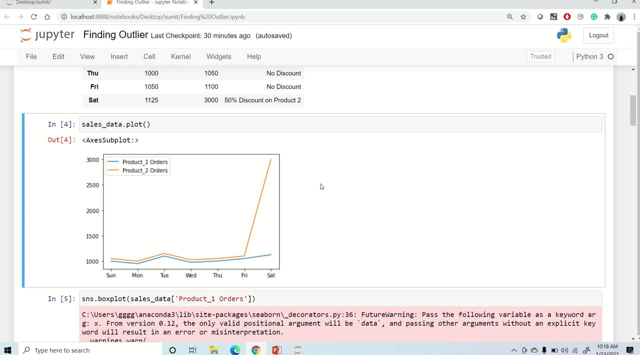 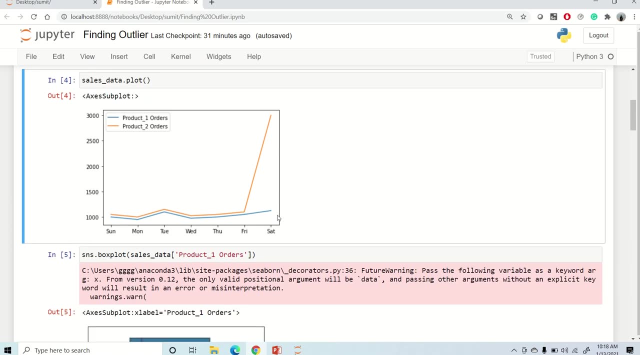 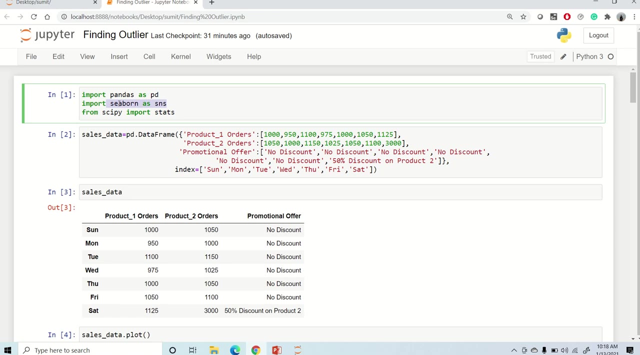 an outlier. so this is the first thing you can do for detecting an outlier. just use plot method okay, and it will see, show you something like this. next go ahead and we can actually plot a box plot. so we are using c bar method for that seaborn library, for that i have imported seaborn here as sns. okay, so if i'll say: 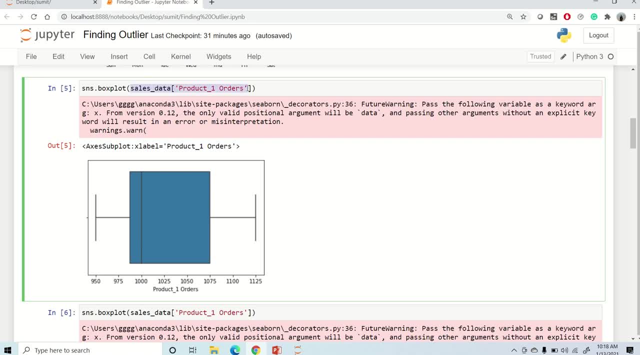 sns dot box plot and i have given the product one orders to plot here. okay, i can see the whiskers and the box here and this is the median line. okay, and this data set is having four quarters: one, two, three and four. this is the interquartile range, q1 and this is q3. right, so this is my box plot and 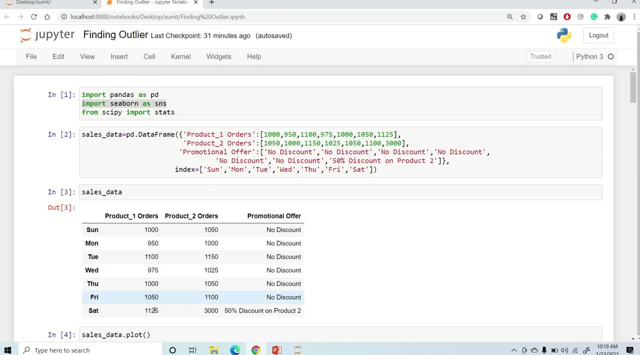 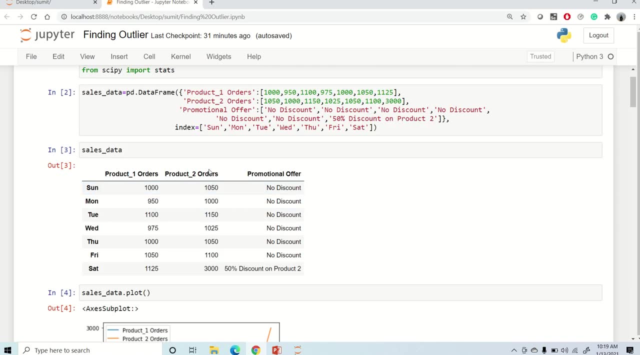 since there is no outlier here. so i am going to plot a box plot here and this is my box plot and there is no outlier in my data set. product one: okay. i, i am seeing this box plot is pretty good. there is no outlier pointed here. but in case of product two orders, there is an outlier, okay. 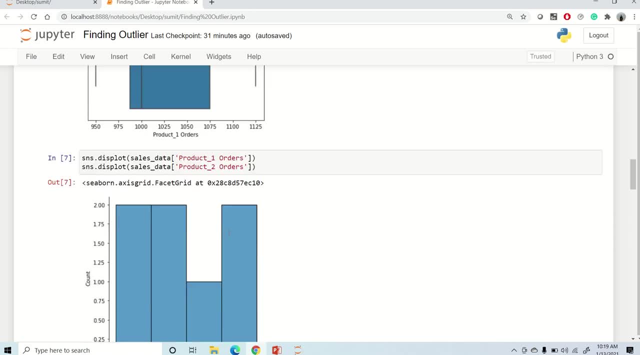 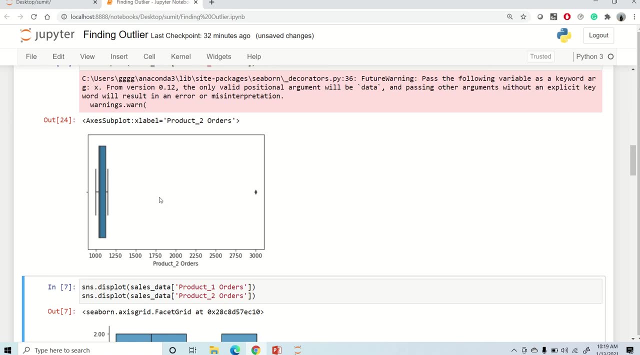 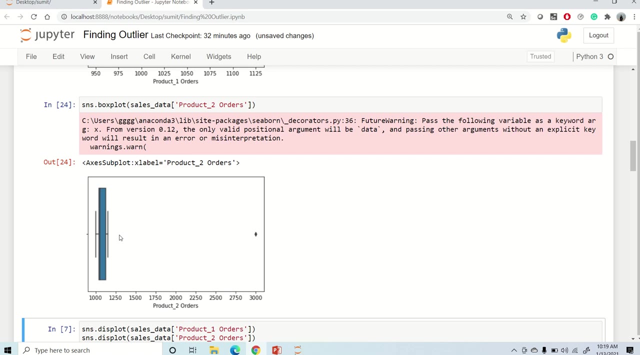 so if you plot box plot for product two, you can see- let me just plot it- this is product one, so i'll say product two. okay, so you can see, this is the box plot for product two and there is an outlier, three thousand from this, far away from this box plot. 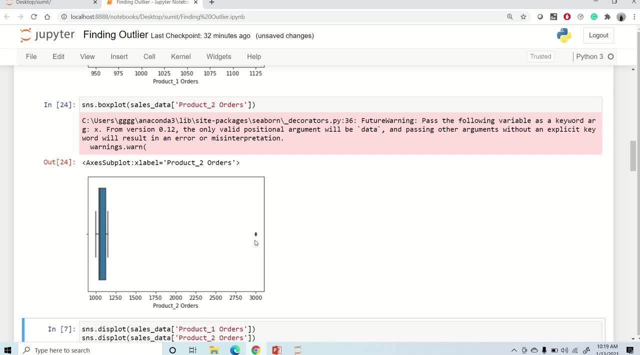 so this is how box plot plots a outlier in your data set. if this value would be like one, two and three, this would have been represented here below the median line. so you can see the difference of box plot without having a outlier and with an outlier. okay, now you can even draw a distribution. 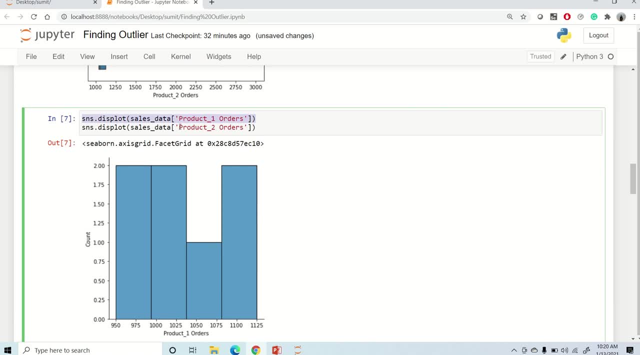 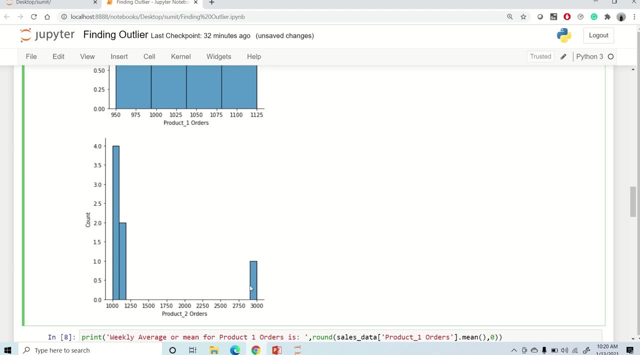 plot. okay, so distribution plot for a normally distributed data would look like this, but for a not normally distributed would look like this: you can see this data point is far away from the others data points. okay, so that is about plotting, and now let's talk about mean and median. so, as i 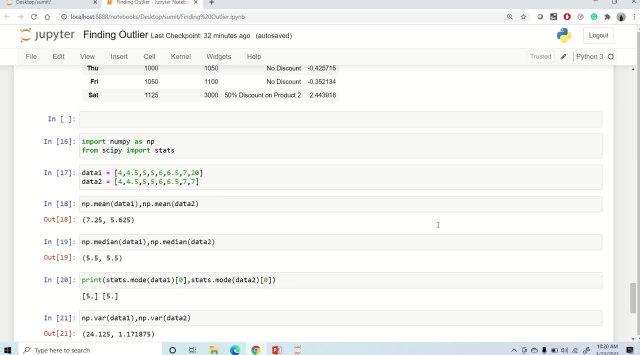 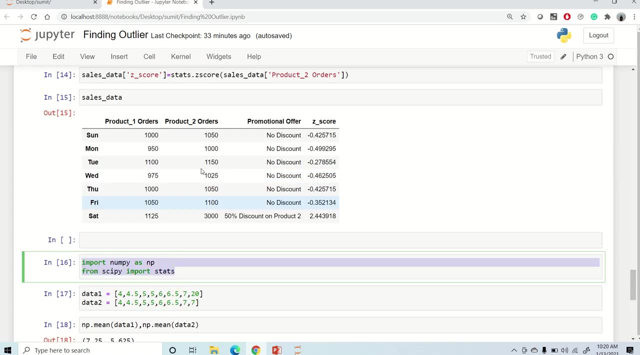 said we can use mean method. we have implemented this using a numpy as well. so if you come below in this stupider notebook, you can see the implementation is done using numpy as well. but this is this implementation is according to panda's data frame. so if you want to find the mean, 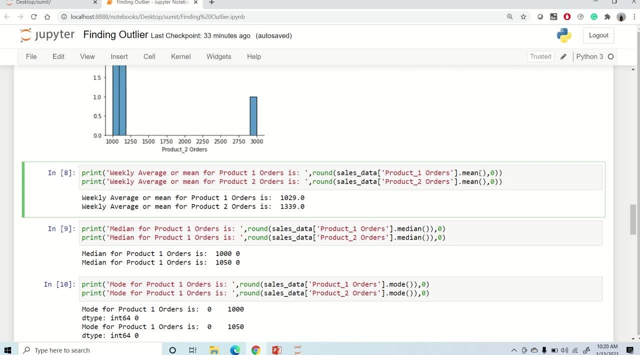 of a data frame. you can use this data frame and you can use this data frame to find the mean of a column in panda's data frame. you can make use of mean method. okay, and you can see. because there is an outlier in product two orders, the mean value is too high. okay, so, as i said, in case there is an. 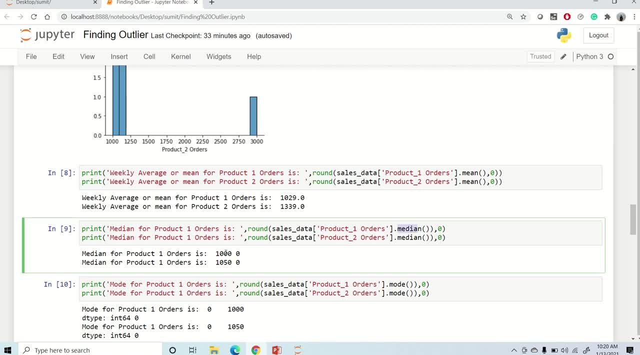 outlier. in your data set you should take median. so i have took median here and the median. in case of both, the data set is similar because median is not affected by an outlier, and so is for mode. even mode is not affected by an outlier. so you can see that the median is not affected by an outlier. 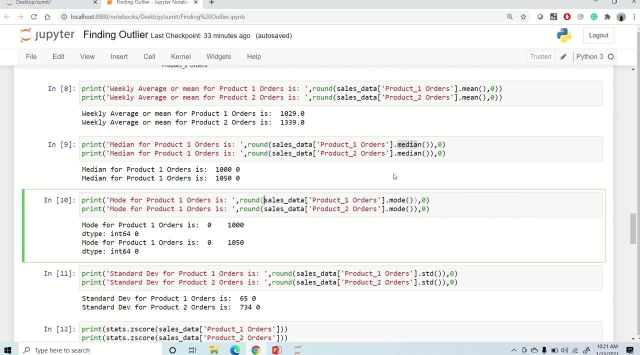 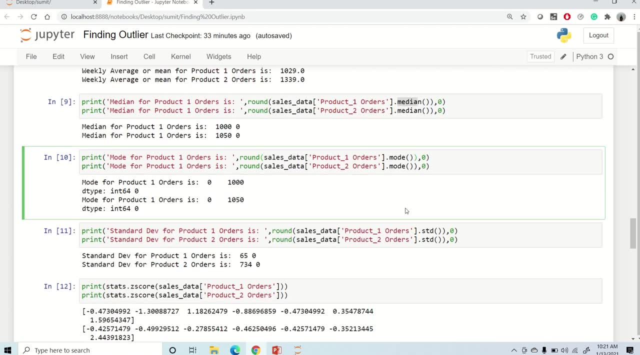 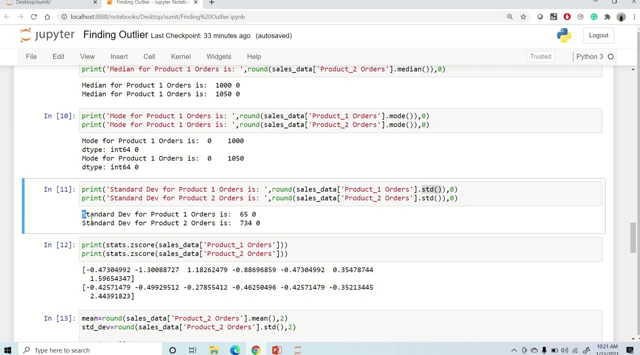 so this is how we find mean, median and mode in panda's data frame: by making use of mean, median and mode method. now, if you want to find a standard deviation, we can make use of std method here and you can see the standard deviation for product. one orders is 65, but since there was an outlier in 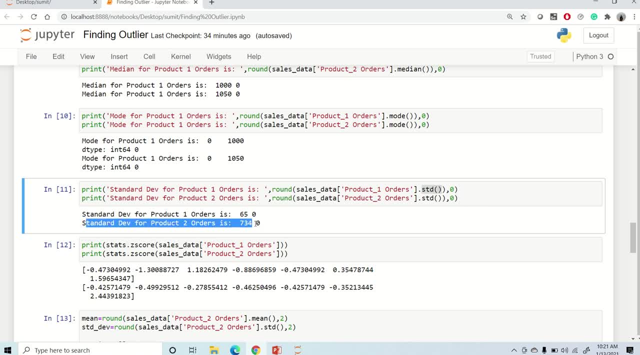 data set 2, the standard deviation is now 734 and please note that a standard deviation is sensitive to outlier, so if there is an outlier in your data set, a standard deviation would increase a lot. okay, so this is what has happened in this case: there was no outlier in data set one. 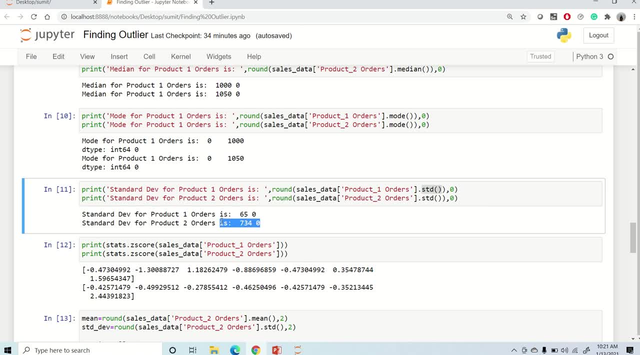 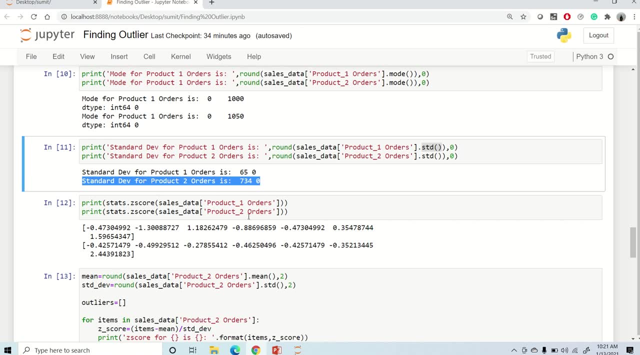 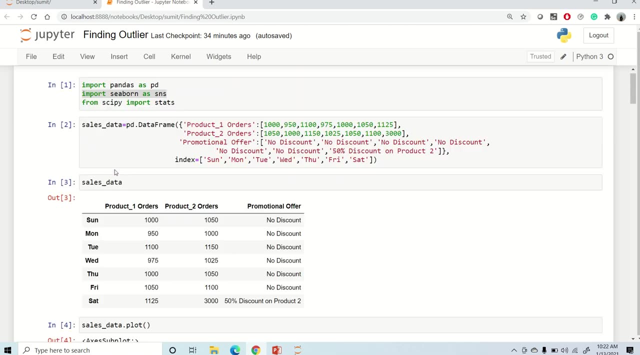 so a standard deviation is 65, whereas there was a standard deviation in data set 2, so it becomes 734, which is too high from the- uh- previous one. okay, now we can calculate z score by making use of states package from the sci-fi library. okay, you can see. 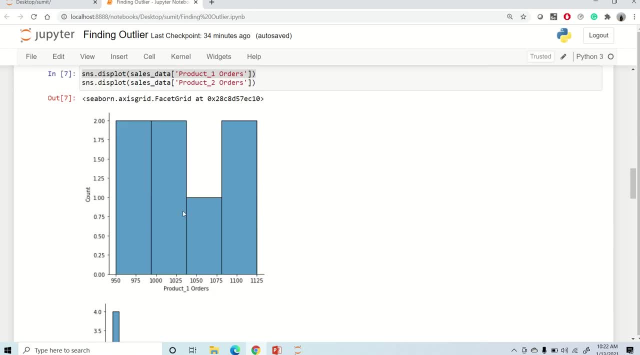 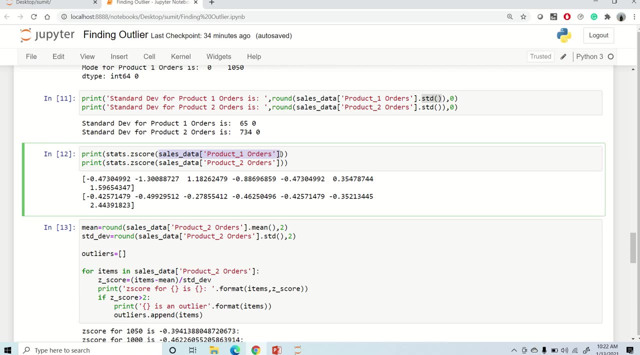 i have imported site estates from sci-fi. okay, so if i'll just say, if i'll just say a states dot z score and provide the column name for which i want to calculate the z score, it will give me the z score for each and individual data point. so i can see: for data point one there is a z score between. 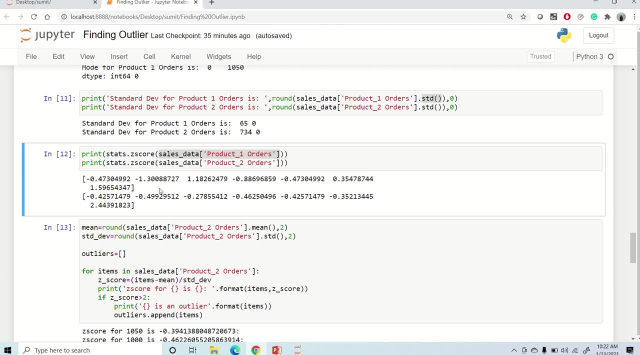 one and uh 0.5 and 1.5. okay, so, as i said that uh for outlier the z score would be around three. so for data point, you can see: uh, the z score for uh this outlier 3000 is 2.44, which is too high, right, so i can. 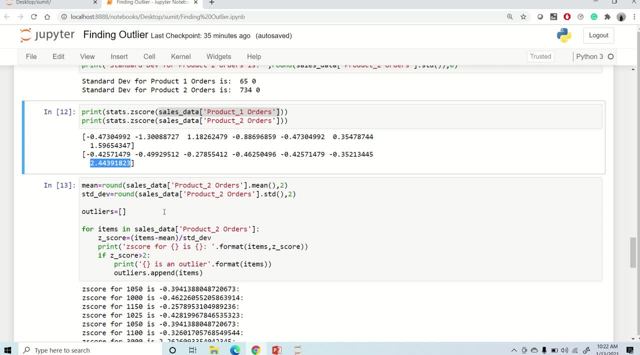 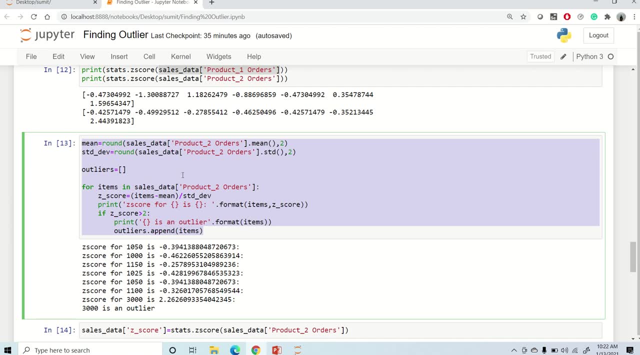 treat this value as an outlier. okay. now, uh, there is just a little bit of code for implementation of outlier detection using panda's data frame. what i have done here: i have took the mean okay, mean of the data set okay and a standard deviation. now, as you know, the formula for z score is this: 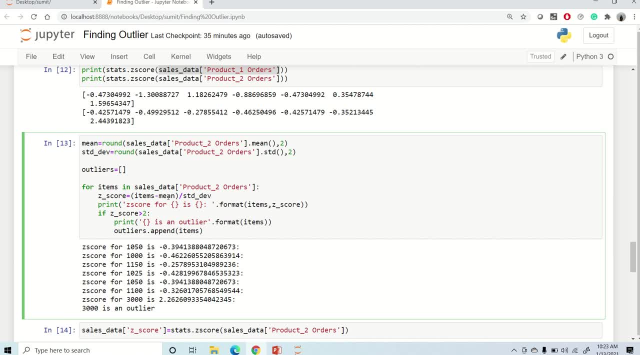 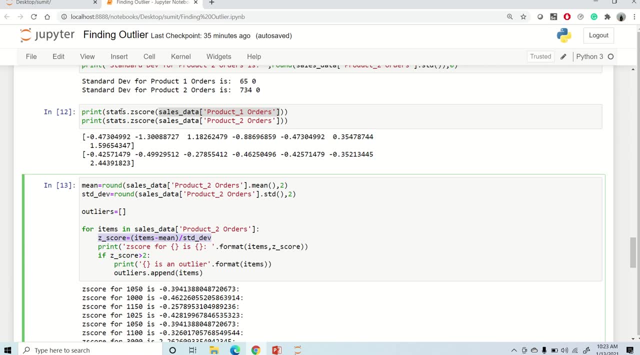 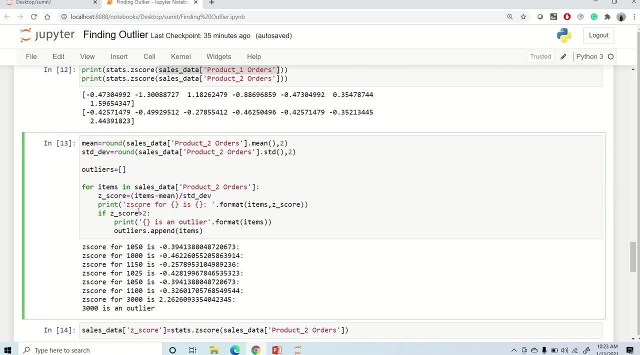 okay, uh, the observation point minus the mean of the data divided by a standard deviation is: this: is what z score. okay, so rather than using a states library here, i can make use of this formula and can calculate z score manually, as i have did in this case. okay, i have even defined a threshold. 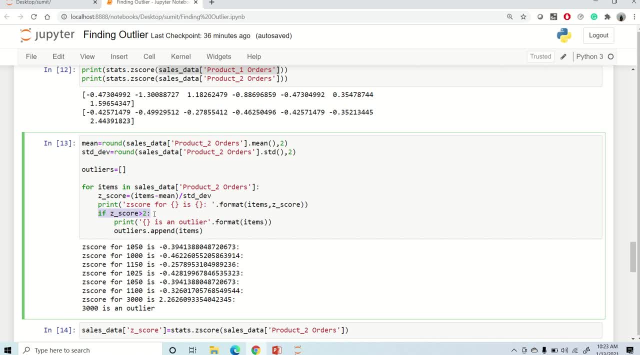 for my business requirement that if z score is greater than 2, treat that point as an outlier. okay, so it is printing for me that 3000 is an outlier. okay, and i store that value in this list. okay, in this list, so outlier dot- append that particular item. okay, so you can use this code for: 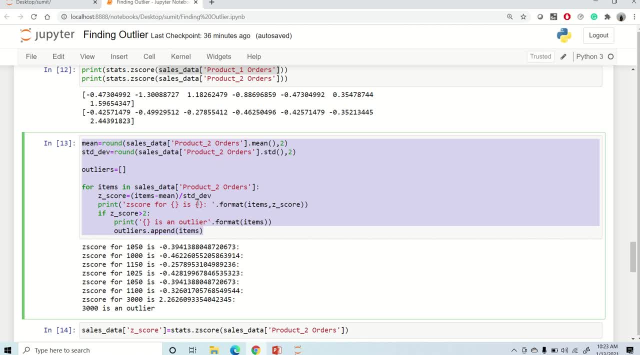 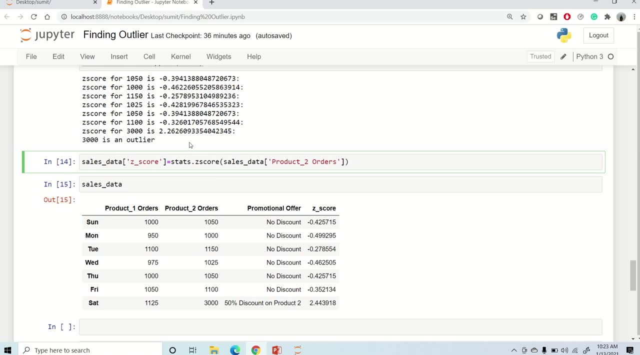 implementation of detection of outlier uh in your code as well. okay, now go ahead and you can even create a new column in your data set for uh, creating z score. so what i have said, i have said sales data, and add a new column called z score and it starts: dot z score, sales data. 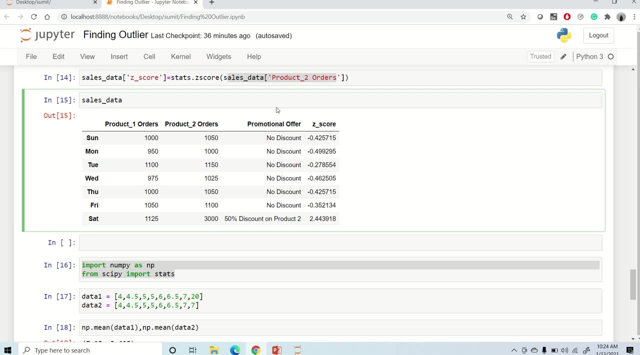 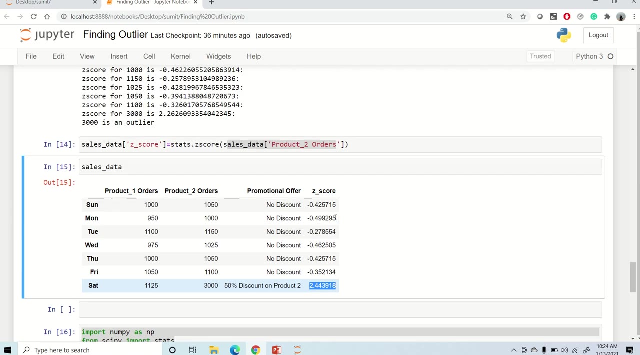 product, two orders, okay, and thereby it added a new column for me which is called z score, and i can see what is the z score for each and individual uh value here. okay, so i can see the z score for this value is 2.44 uh, by a stats package, okay, which is bit different from the one which we 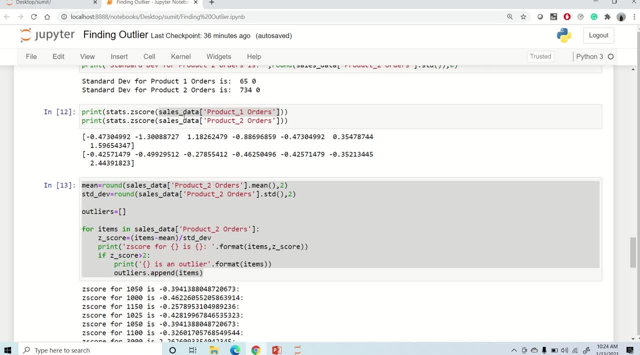 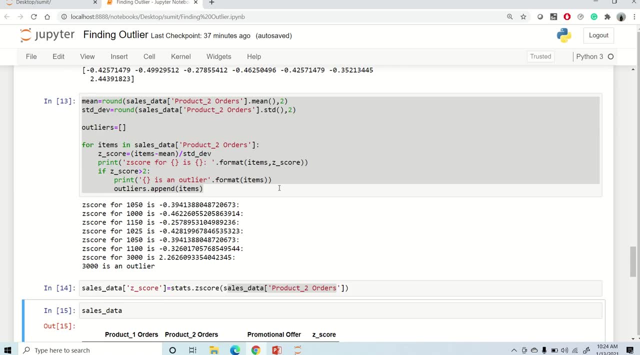 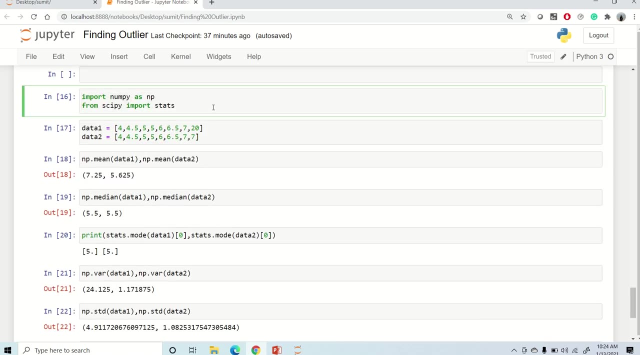 have calculated. that is because of the uh value. we are taking uh after decimal points. okay, so this is an outlier and this is uh the whole thing about implementation of outlier detection using z score and box plot using pandas data frame. but we can do the same thing using numpy.